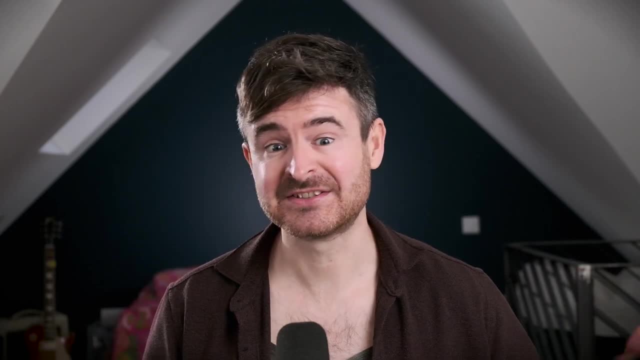 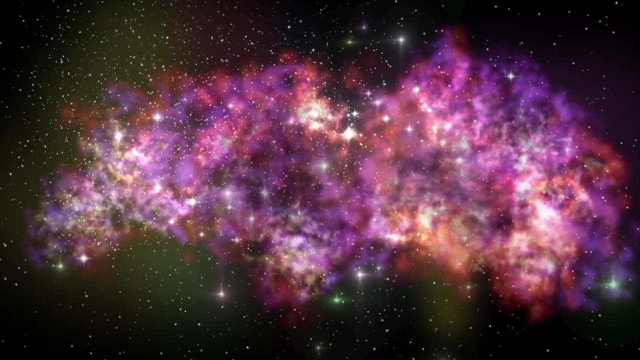 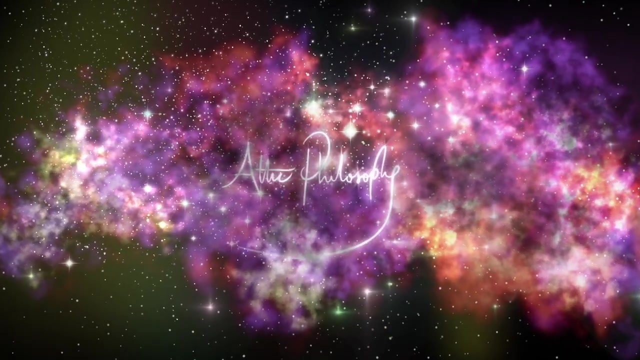 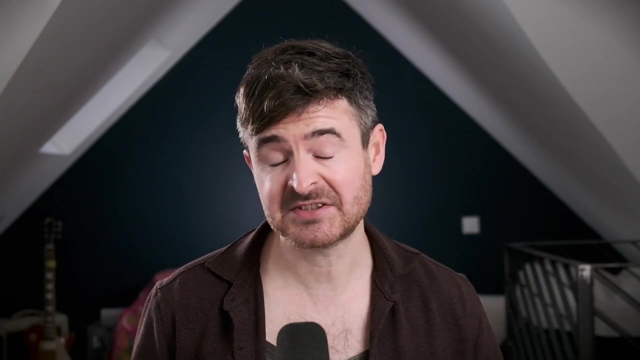 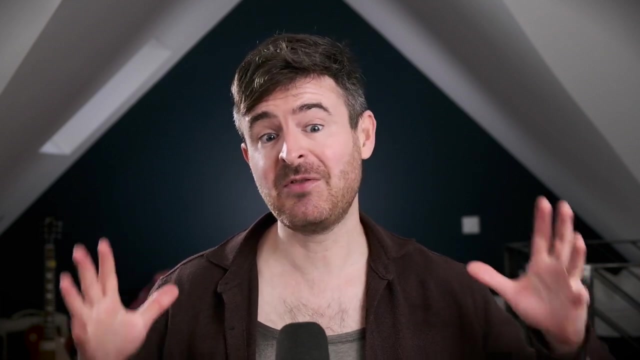 How do these ideas of soundness and completeness relate to the tree test in logic? Let's find out. Hi guys, welcome to The Attic. My name's Mark Jago. I'm a philosophy professor in the UK. Recently on the channel we've been talking about proving things in logic using the tree test. 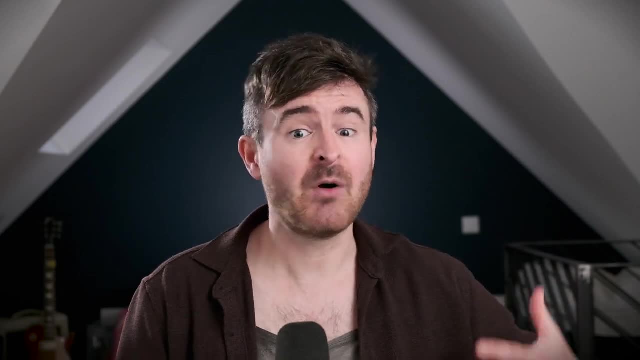 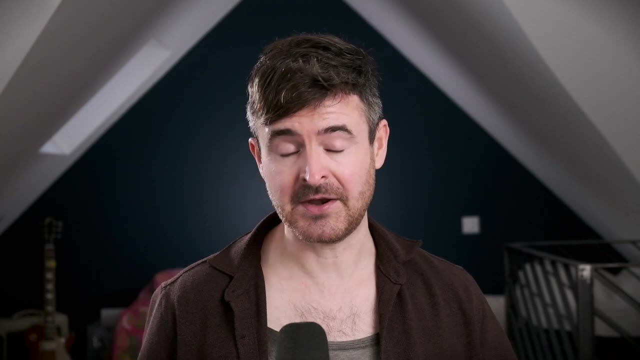 And then in the last couple of videos, I've been talking about the ideas of soundness and completeness. okay, So if you're unsure about what they are, have a look at the previous video. In this video I'm going to be thinking about how those general ideas of soundness and completeness 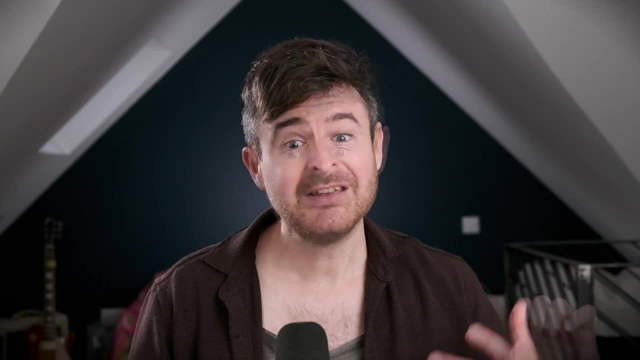 relate to the tree test specifically, So this is a really useful story. I'm going to be talking about how soundness and completeness relate to the tree test. It's a step to think through before we get into the nuts and bolts of proving soundness, and 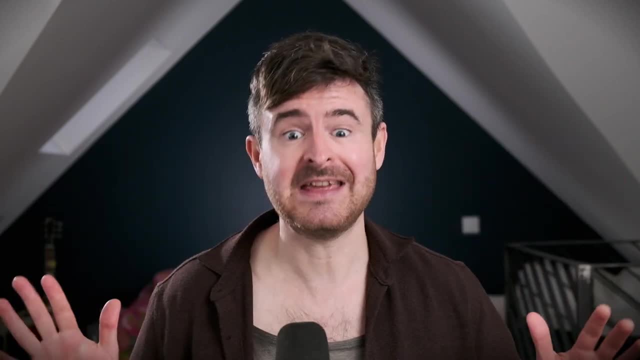 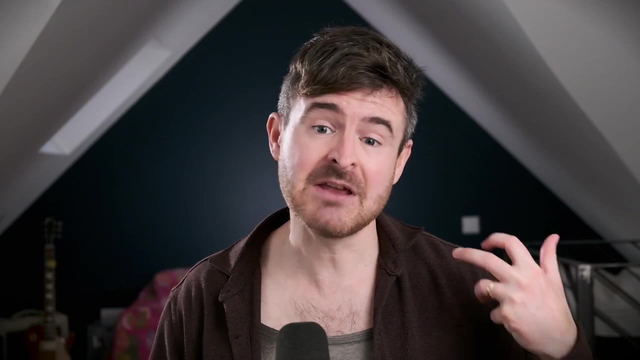 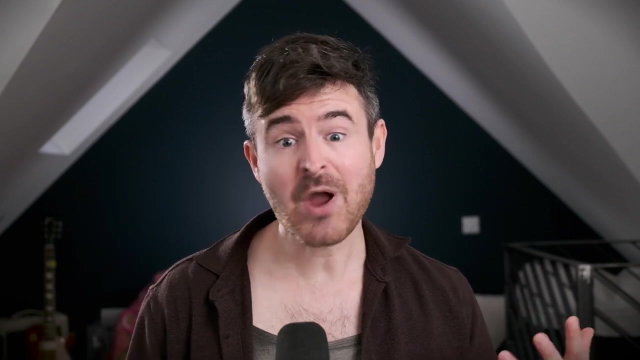 completeness. So we're going to be manipulating our idea of soundness and completeness to make it fit specifically to the tree test, And that will actually make the process of proving soundness and proving completeness much easier. Okay, so if that sounds good to you, you can do me a favour. 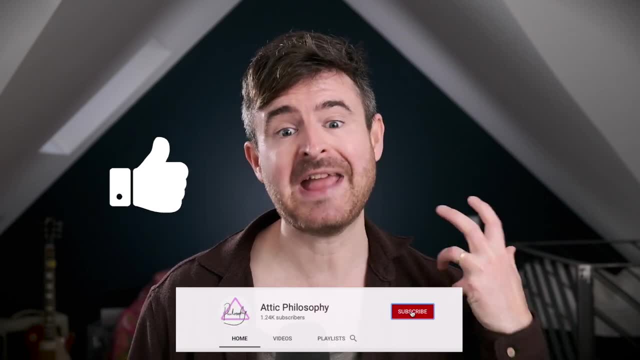 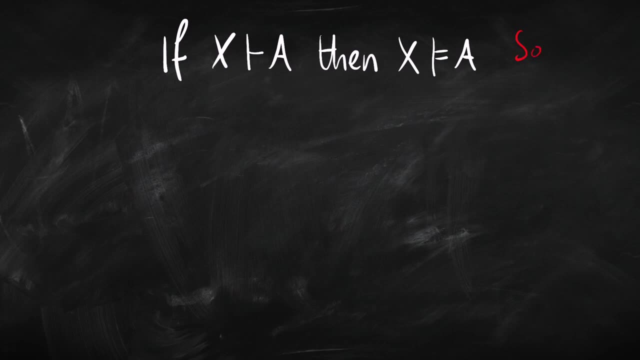 before we get going, Give this video a thumbs up. That really helps it reach more people out on YouTube, And if you're liking this stuff, why not subscribe to the channel? Okay, so here we've got soundness. We went over what this means in the previous video. 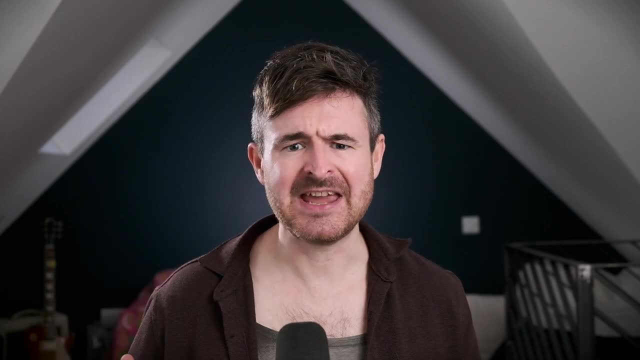 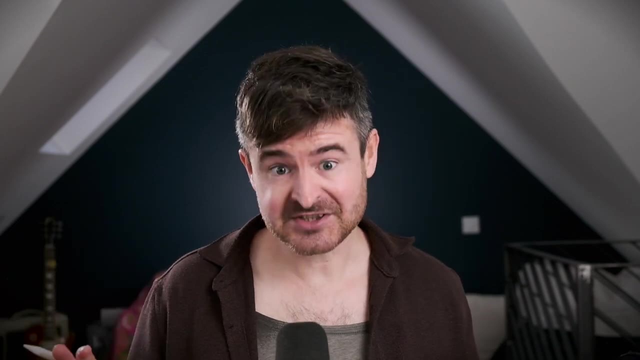 What I want to do is start manipulating this statement in a way that's going to make it easier to prove before we actually get to the proof. So the first step we're going to take is a completely general step. We would probably do this, whichever proof system we're thinking. 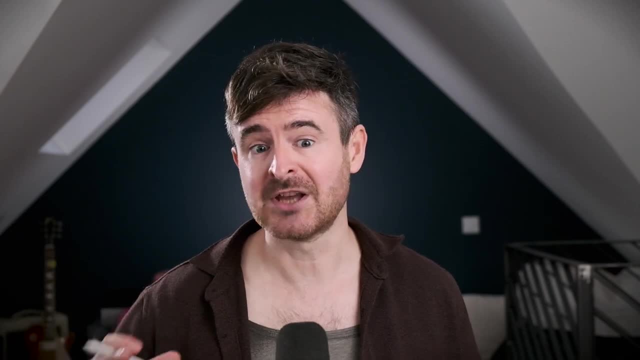 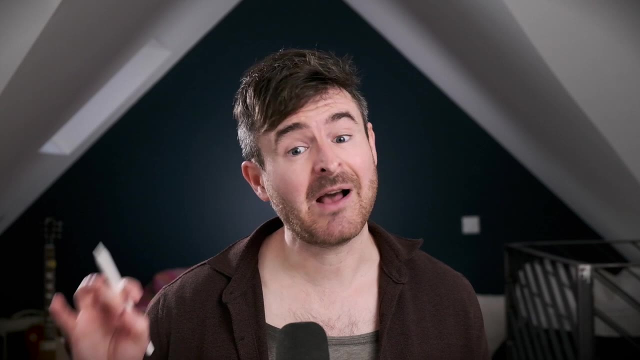 about. So, whether we're thinking about you know natural deduction, we're thinking about you know trees or whatever, and whichever logic we're thinking about, this is a really good step to take. I'm going to go through it thinking about soundness, but very much the same applies to 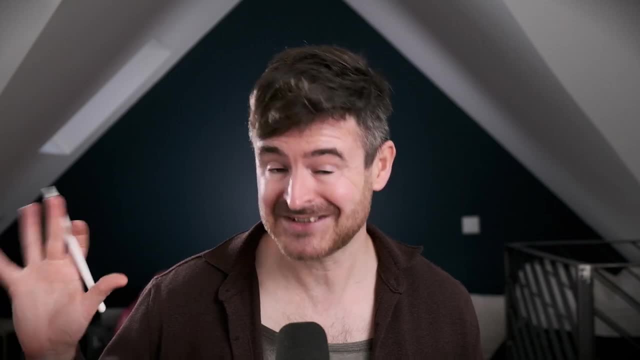 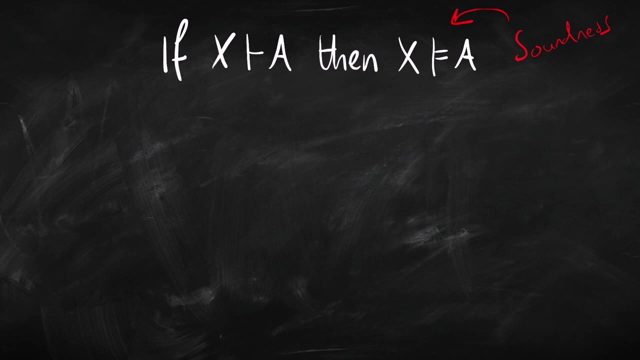 completeness, just with the converse if-then statement. Okay, so we've got this if-then statement of soundness. It's usually a really good idea to think about proving the contrapositive. So what do I mean by the contrapositive? Well, if we have any if-then statements, 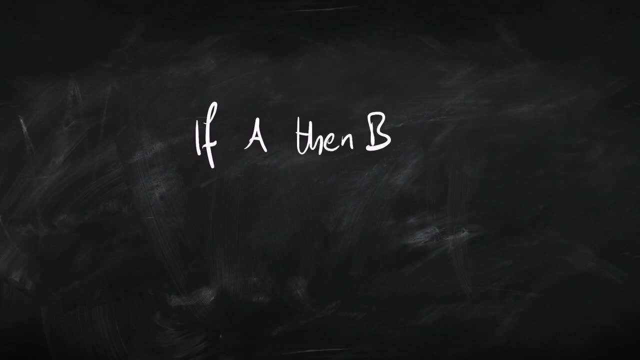 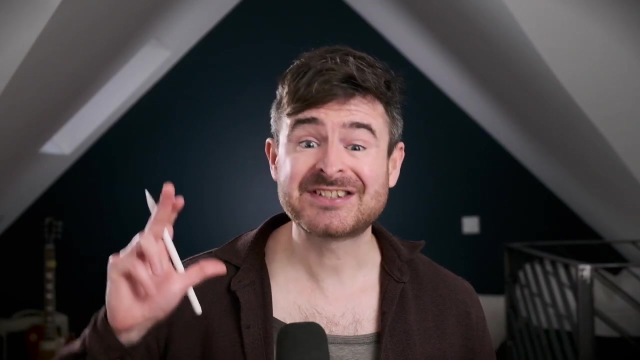 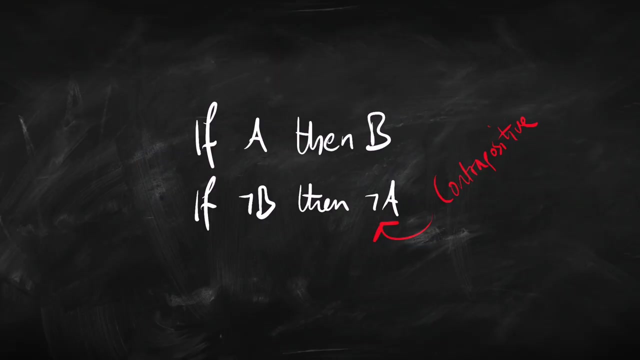 if A then B. its contrapositive goes like this: if not B, then not A. Okay, that is the contrapositive of the original if-then. So we've got to be careful to distinguish the contrapositive of an if-then from the converse of an if-then, The converse of if A then B. 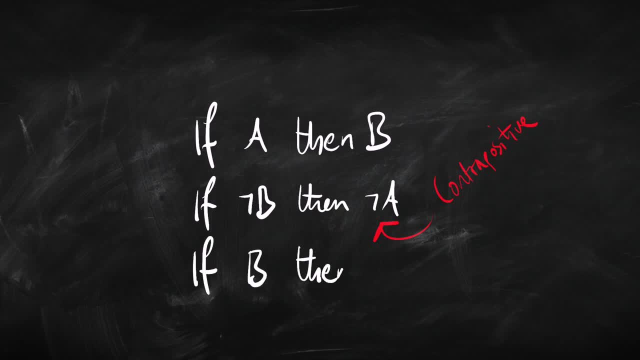 just goes. if B, then B, Then A. Okay. so the contrapositive is the one that adds negations, whereas the converse just switches around the order of antecedent and consequent Okay. so if this is soundness. 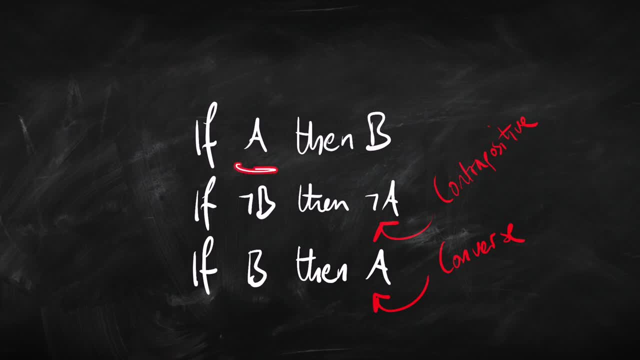 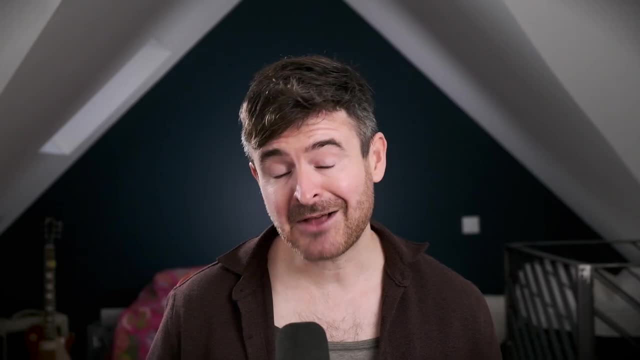 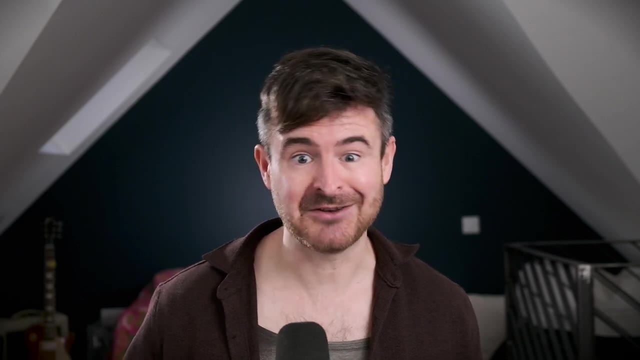 this would be completeness. right? If this goes from proof to truth, then this one would go from truth to proof. So soundness and completeness are converses of one another. So that's not what we want here. We don't want to be jumping from soundness to completeness, or? 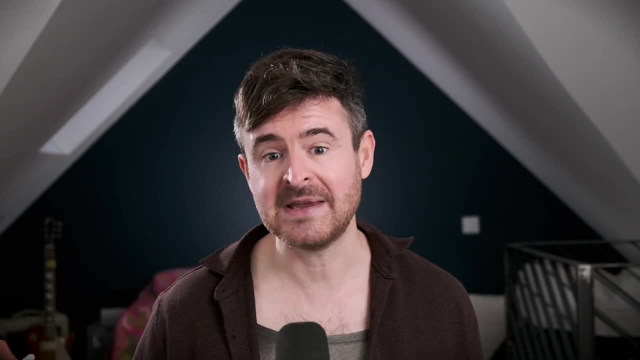 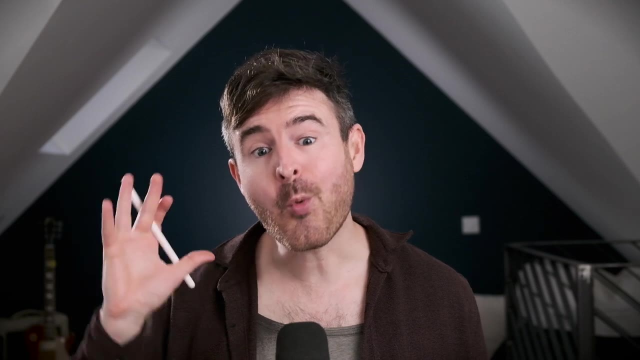 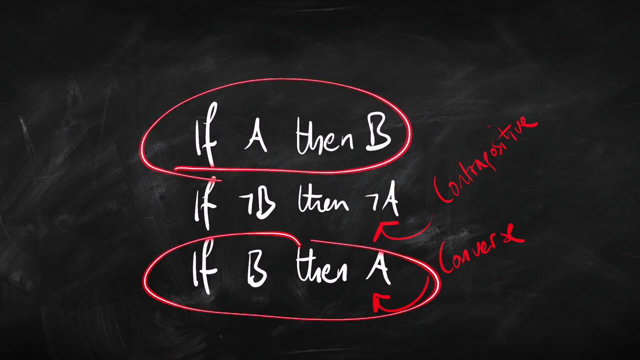 whatever, We want to focus on one of them, either soundness or completeness, And what we want is a way of manipulating that statement that keeps it equivalent but that makes it easier to get at and start proving Clearly the converse of a conditional isn't going to be equivalent to it. 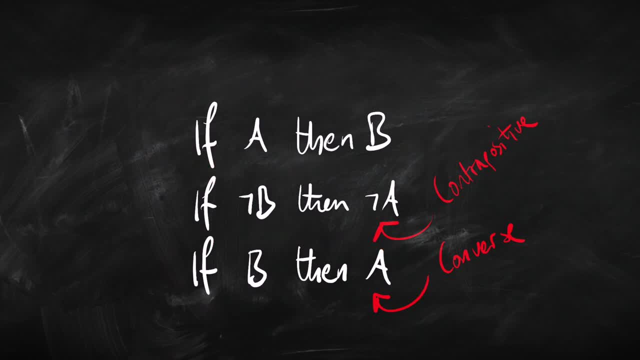 If A then B means something very different from if B then A, And it might often be that one's true and the other's false, But a statement like this and it's contrapositive always have the same truth conditions: They're equivalent to one another. 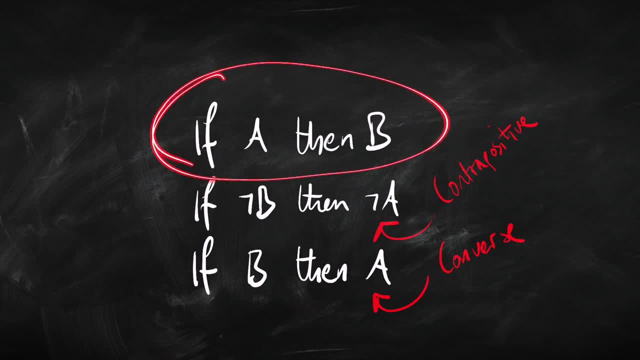 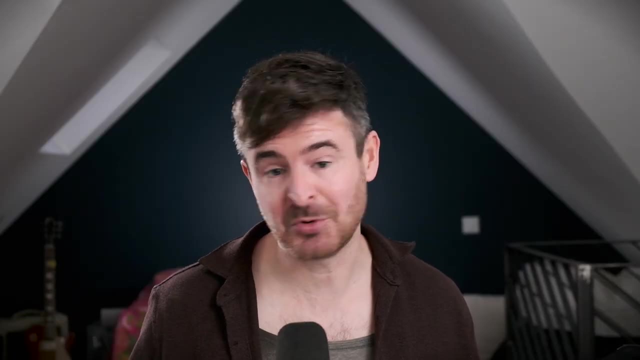 In the simple case of true functional logic. just think about what the truth table for this looks like. It rules out the case when A is true and B is false. This rules out the case when B is false and A is true, So they've got the same truth table. That's why, in the simple case of true, 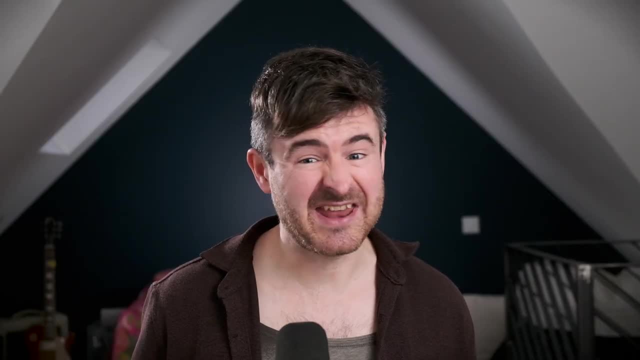 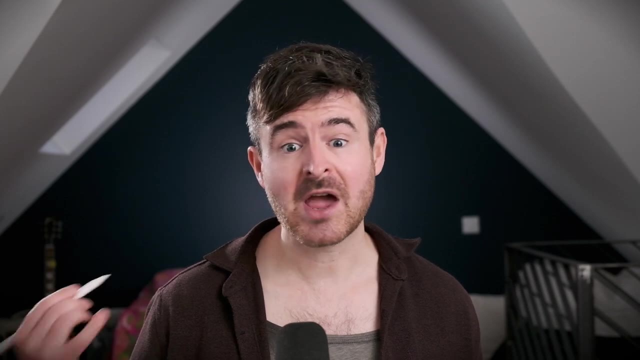 functional logic, they're equivalent. So if A is true and B is false, they're equivalent. But pretty much they're going to be equivalent in whatever logic we're looking at. So pretty much whenever we're trying to prove soundness or completeness, we're going to do as the first step 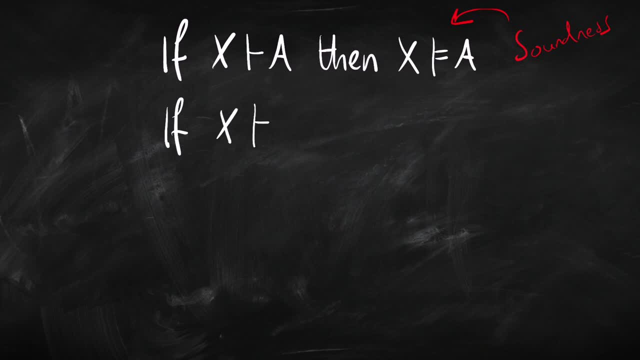 taking the contrapositive. So in the case of soundness that would go like this: Okay, so here I'm writing a line through the symbol, like a kind of a slash through the symbol to say it doesn't hold. So this symbol means entailment. So here I'm saying the entailment. 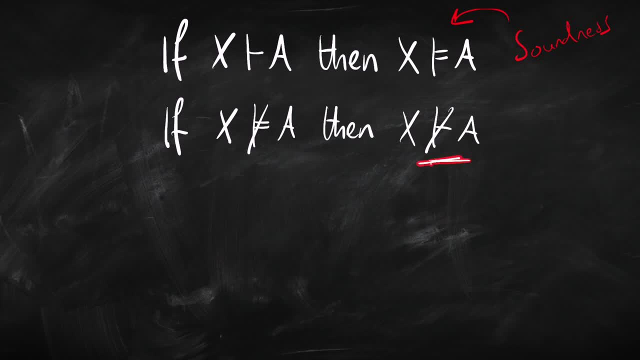 doesn't hold. So here I'm saying the entailment doesn't hold. So here I'm saying the entailment doesn't hold. This symbol means a proof. So here I'm saying we don't have a proof, The proof doesn't hold. 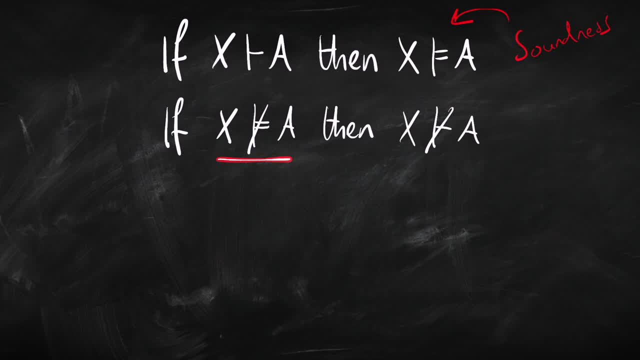 So what the contrapositive of soundness is saying: if we don't have an entailment from X to A, then I can't prove it. Okay, that pretty obviously means the same thing as soundness, right? If I prove it, then it's true. So if it's not true, then I can't prove it. I can't prove anything. 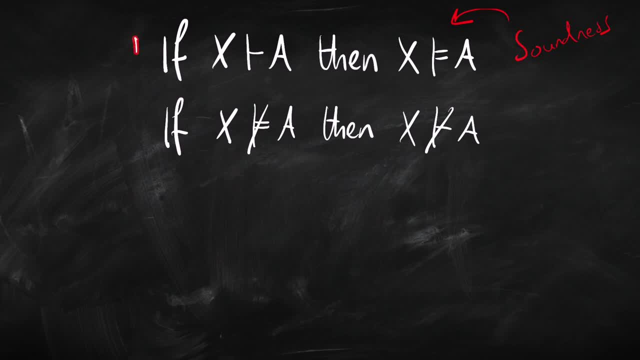 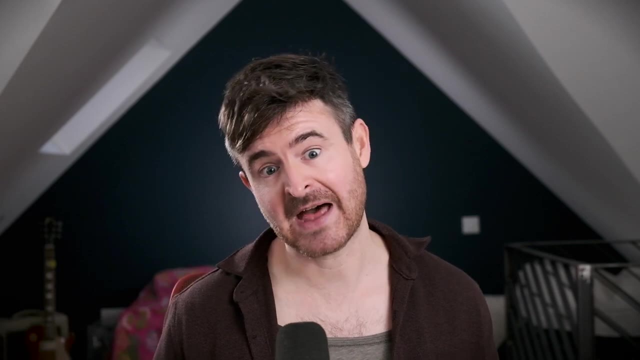 that's not true. So if I do prove it, then it is true. So these are equivalent. But it turns out that it's much easier to prove this form of soundness than it is to prove this. And the same holds for completeness, right? If we're trying to prove completeness, that is, if we've 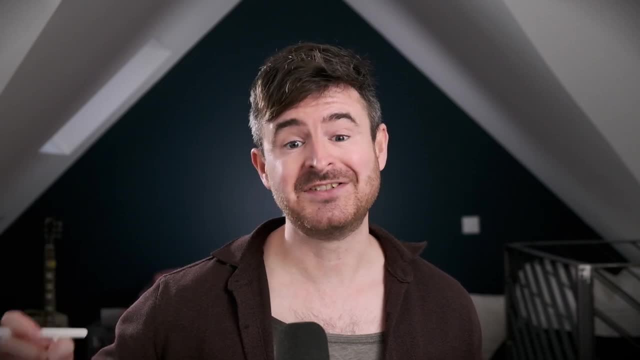 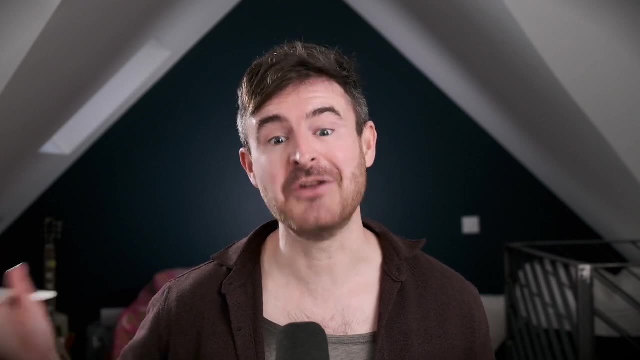 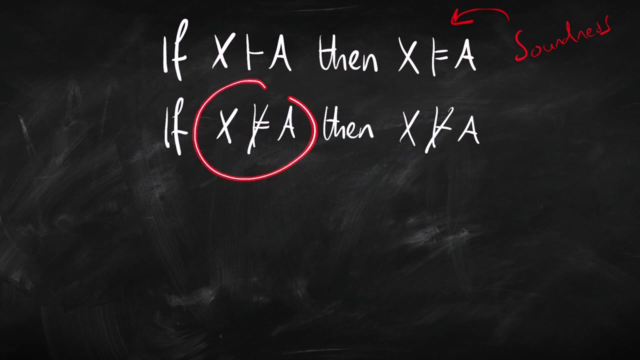 got a genuine entailment, then we can prove it. What we're going to want to do is prove the contrapositive, That is to say, if we can't prove something, then it's not a genuine entailment. The next step in manipulating these kind of conditionals is: we're going to think: 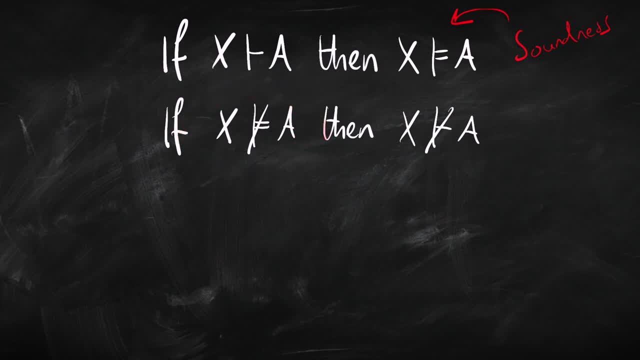 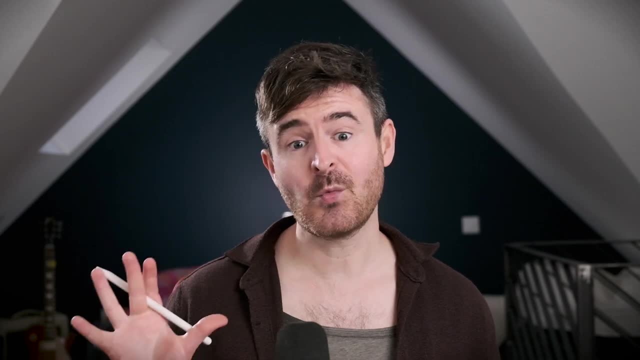 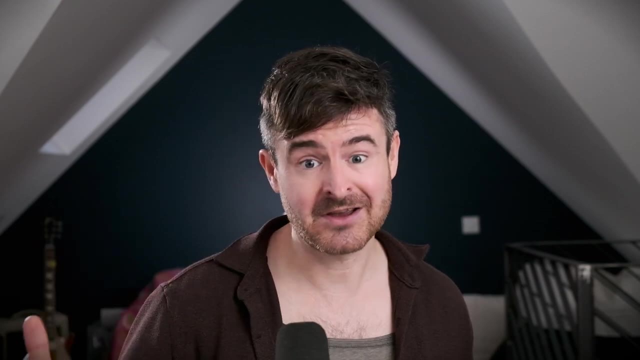 what this means. So I just said that this means we don't have a genuine entailment from the premises X to the conclusion A. But there's different ways that we can say that, And a helpful way to say it in the context of soundness or completeness is by putting it in terms of satisfiability. 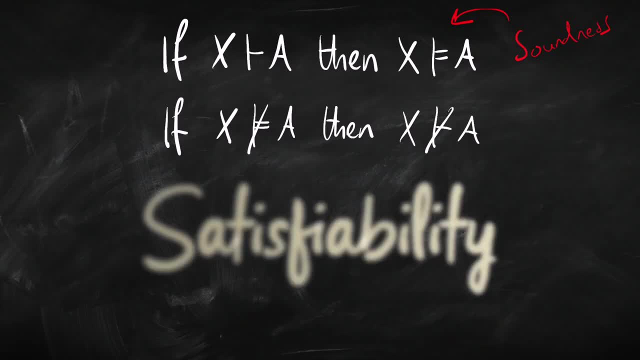 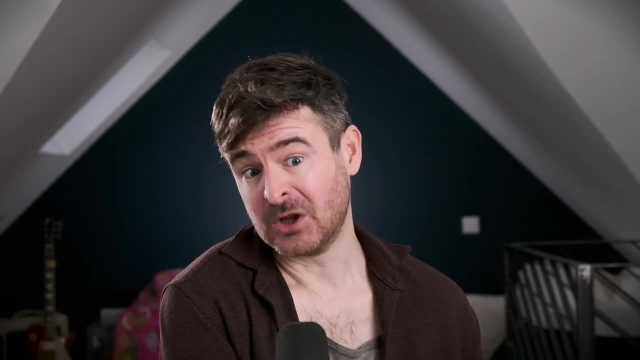 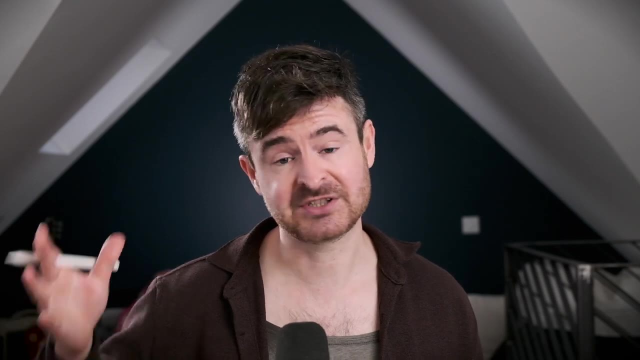 So basically, to say that something is satisfiable kind of means it can be true. Okay, so a sentence is satisfiable if, from the point of view of our logic, it can be true. So if we're in propositional logic, that would mean some valuation assigns true to it. If we're in the 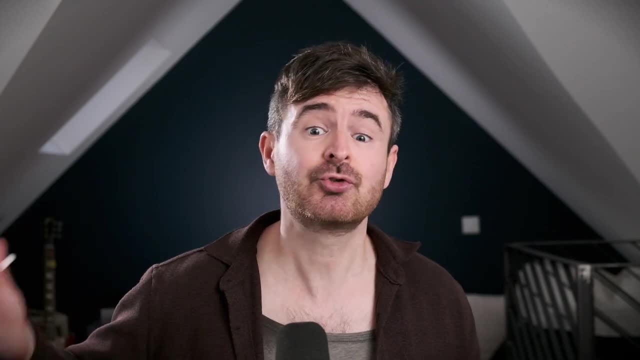 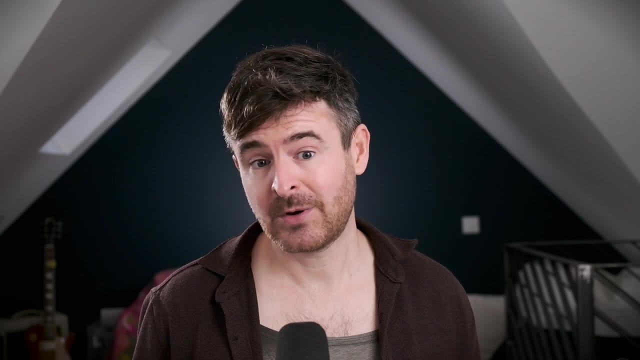 context of first order logic, that means that that sentence is true in some model or other. Okay, some model satisfies that sentence. We might also be talking about sets of sentences, And this is where it gets a bit more interesting. A set of sentences is: 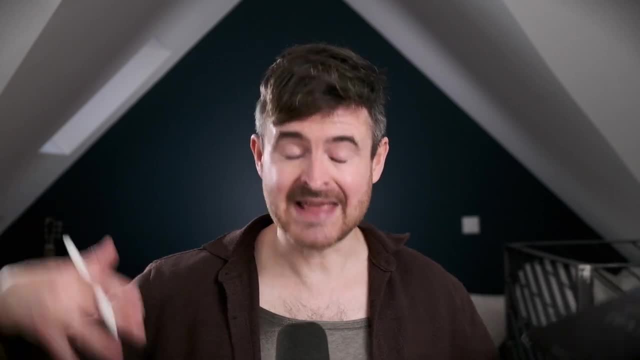 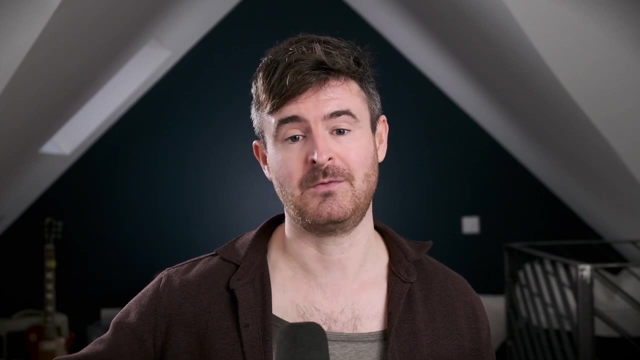 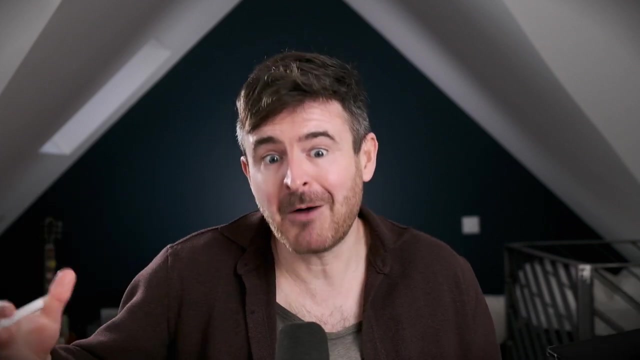 satisfiable if they can all be true together. from the point of view of the logic: Okay. so in propositional logic that means that some valuation makes them all true. In context of first order logic, it means they're all true in one model. Okay, so some model makes all of them. 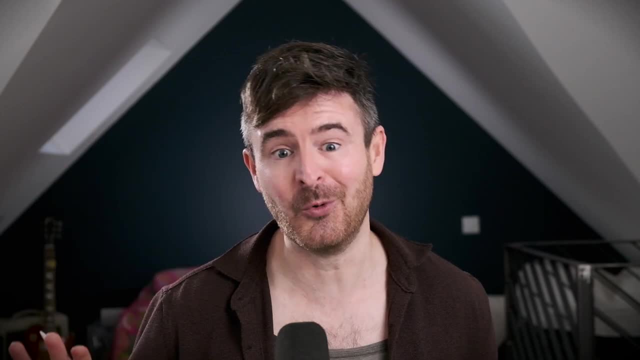 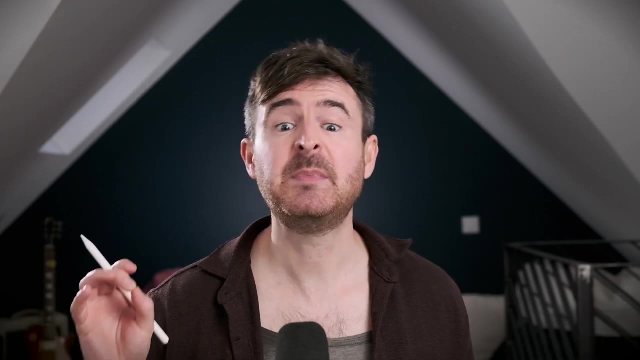 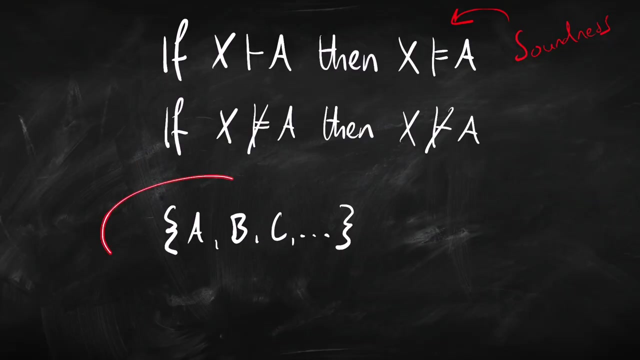 true. at the same time, Some model satisfies all of those sentences. Now, the reason we're focusing in on satisfiability and unsatisfiability is because there's an interesting relationship between satisfiability and entailment. Let's see how it goes. Here's a. 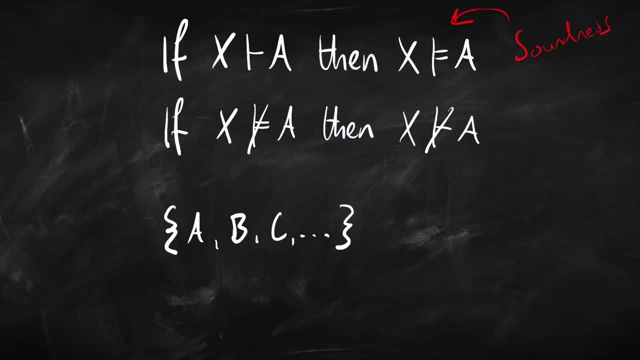 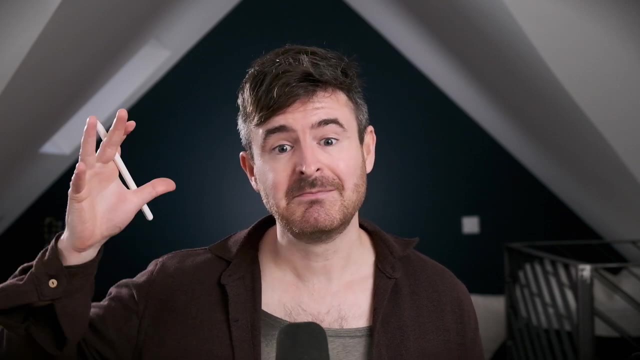 set of sentences A, B, C and so on. Let's suppose that it is satisfiable. Well, that means all of those sentences can be true together. Okay, so some valuation or some model, depending on whether we're talking about propositional or first order logic is going to make all of those sentences. 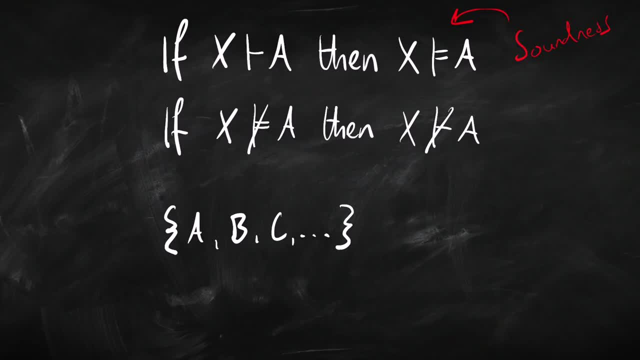 true at the same time. So let's focus on propositional logic. We've got valuation. let's say that V satisfies this set of sentences. It makes all of them true. So in particular, it makes A true. So what's it going to say about not A? Well, if that valuation 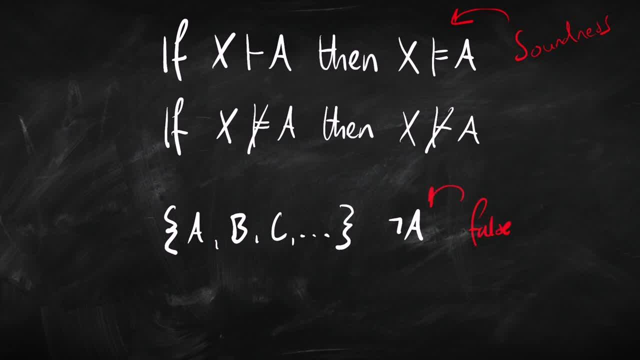 makes A true, it's going to make not A false. Now, what that's going to mean is that those other sentences in the set that we started with B, C and so on- don't entail not A. Why is that? Well, we just say that A is true. So what's it going to say about not A? Well, we just say that A is true. So what's it going to say about not A? Well, we just say that A is true. So what's it going to say about? 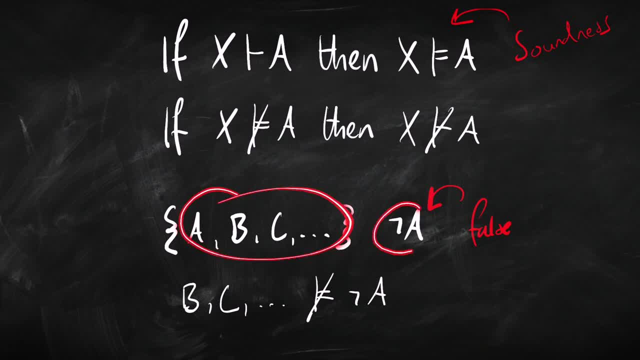 that. Well, we just say that A is true. So what's it going to say about not A? Well, we just say that some valuation makes all of these true, so makes that one false. So, in particular, some valuation makes those true and that one false, right, And if something makes those true but that false, 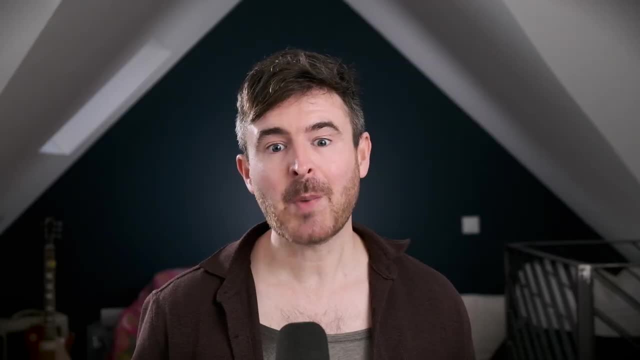 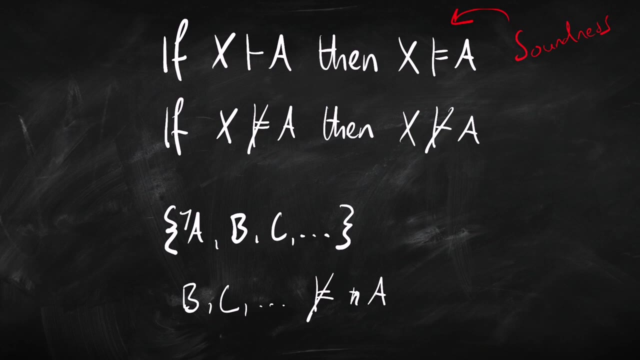 then they don't entail that. Now suppose we swap A for not A. So let's just put in a negation here and let's take out a negation there, because basically a double.